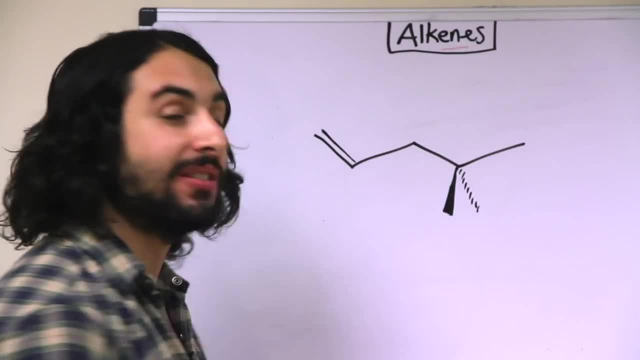 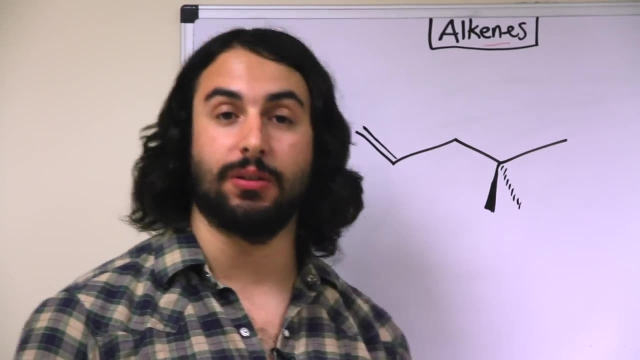 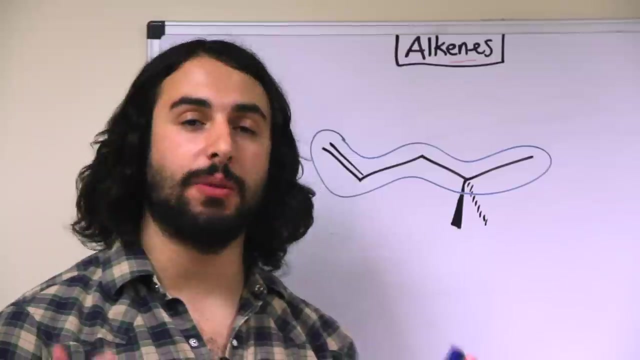 "-ene" to let us know that there is a double bond present in the molecule. Now, fortunately, most of the rules remain the same. We're going to identify the longest carbon chain and, just as with the presence of the hydroxyl group, the presence of the double bond means that we're going to number. 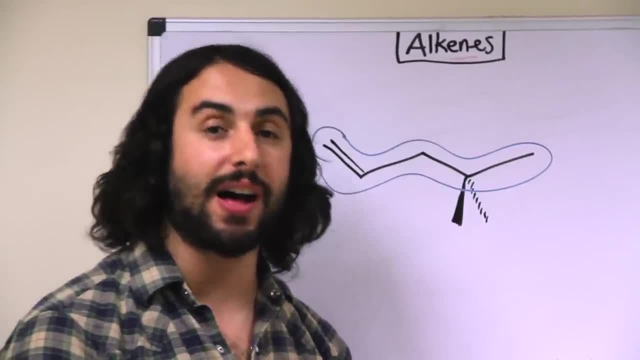 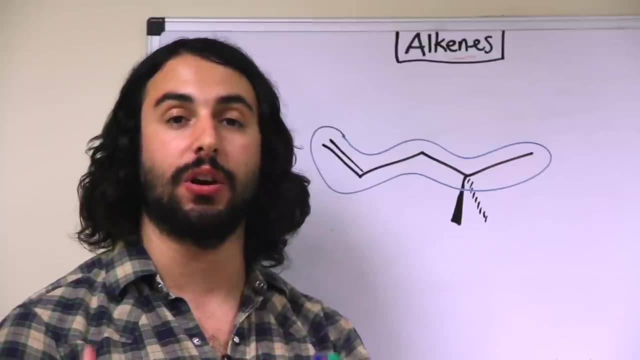 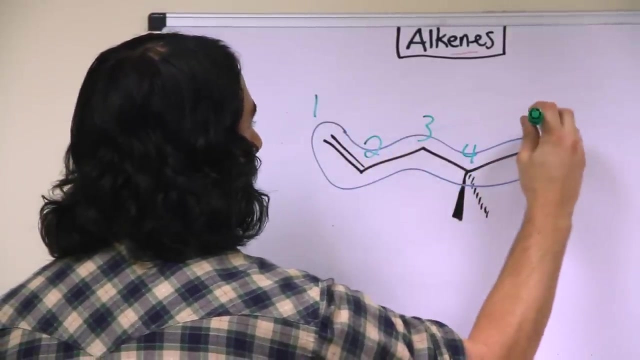 the parent chain so as to give the double bond specifically occurring soonest, even if there is some alkyl or halogen substituent occurring sooner if we number from the other side. So here we're going to need to number left to right. So let's identify that there are two methyl groups over. 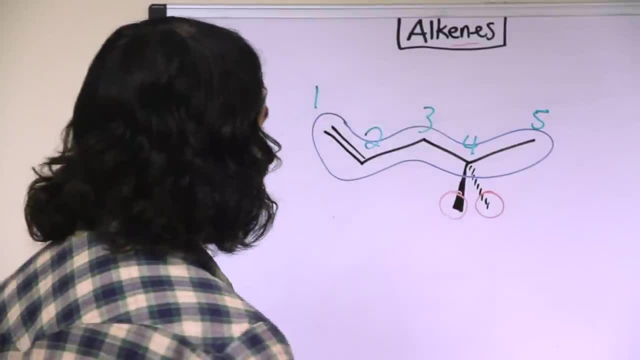 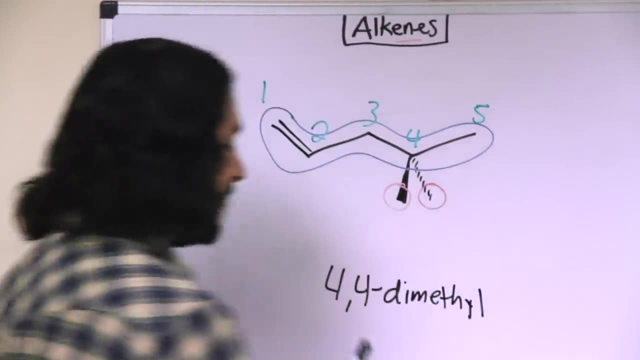 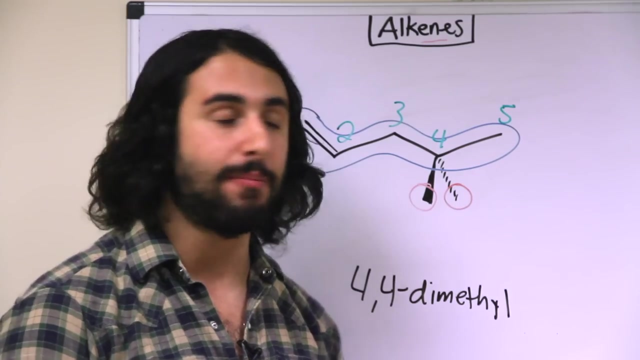 here on carbon four. So we are going to list that first in the molecule That's 4,4-dimethyl. We do need to list both of those, otherwise there would be ambiguity as to where the second methyl group would be, So 4,4-dimethyl. 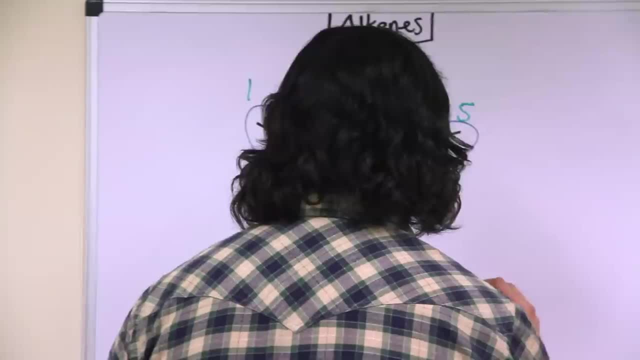 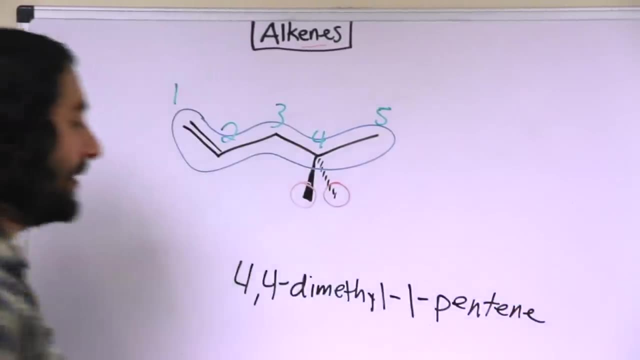 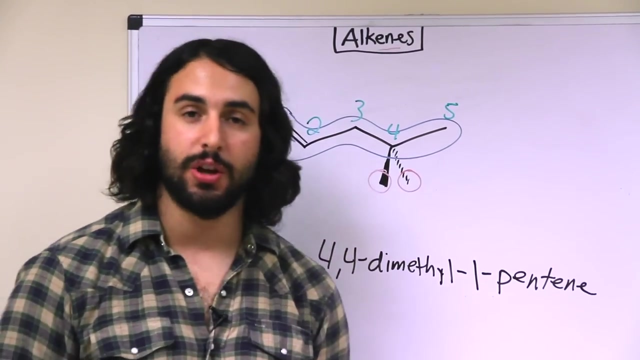 and then we have to list the location of the double bond It occurs. it begins at carbon one, so this is 1-pentene, So 4,4-dimethyl 1-pentene. We do need to list where the double bond occurs in the molecule so as to remove ambiguity as to its location. 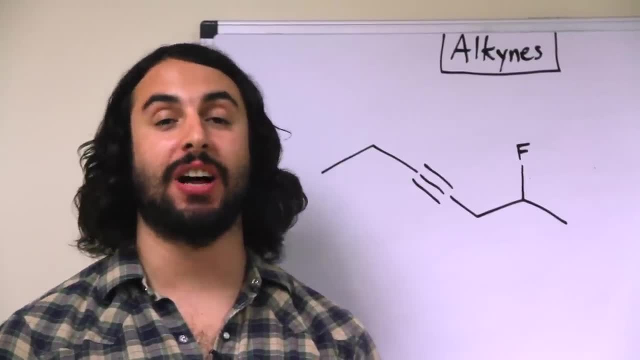 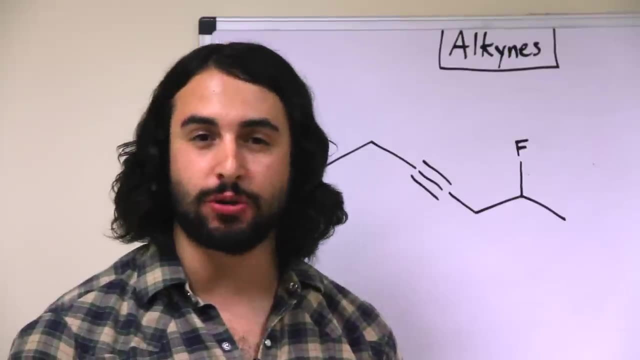 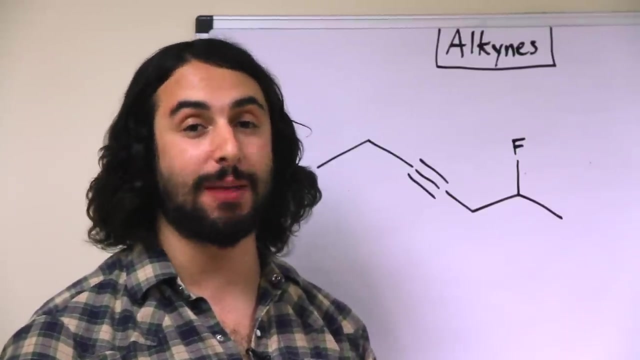 So let's take a look at alkynes now. An alkyne is a hydrocarbon that contains at least one triple carbon-carbon bond. Now alkynes can be a little bit tricky to draw properly, because any carbon atom that is participating in a triple bond is necessarily sp-hybridized. This means that it exhibits: 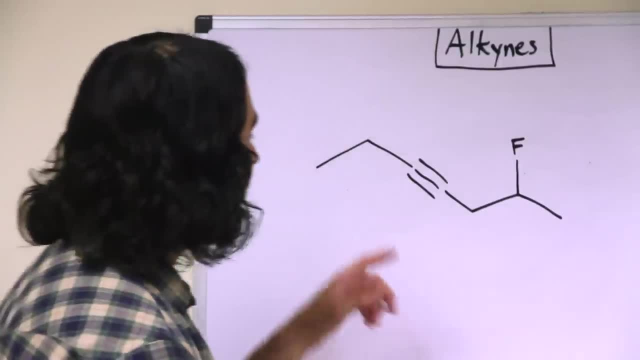 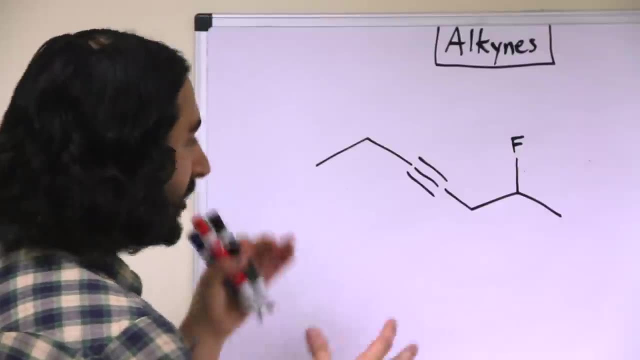 linear molecular geometry, if we remember from gen chem, and that means that the two carbons that it is attached to must be 180 degrees apart. So this looks a little funny, but bear in mind that these are carbon atoms and these are the two carbon atoms that are participating in the triple bond. 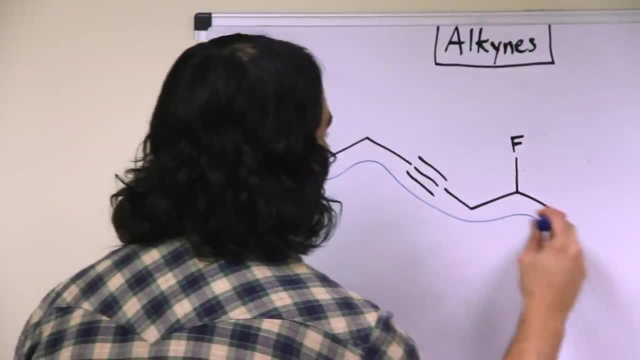 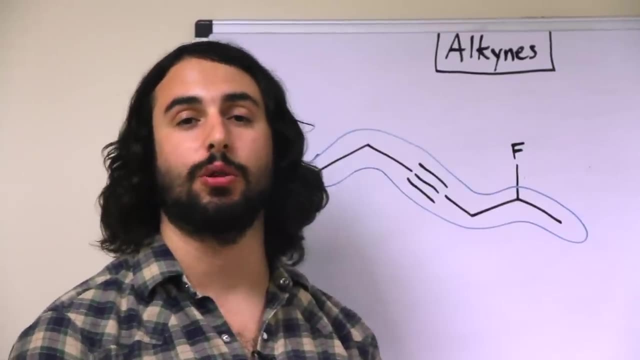 So let's go ahead and circle the longest chain. Now we have to number it and, as you would expect, just as with the double bond or the hydroxyl group, we must number this so it's not sp-hybridized. Now we have to number it and, as you would expect, just as with the double bond or the hydroxyl group, we must number this so it's sp-hybridized. 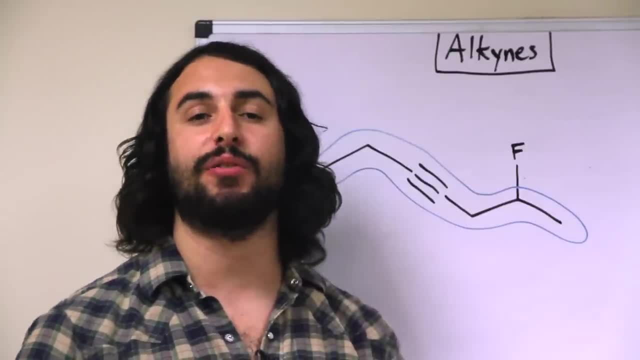 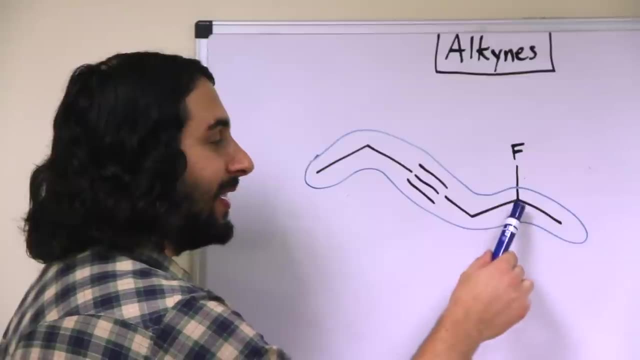 as to give the triple bond occurring soonest, even if there is some other alkyl or halogen substituent occurring sooner from the other direction. So that means that even though a fluorine is on carbon 2 coming from the right side, we must number this from the left, because 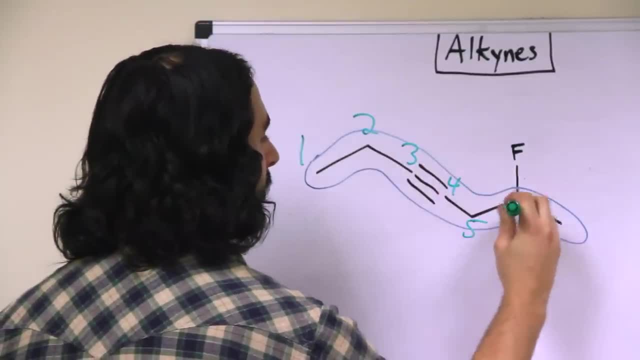 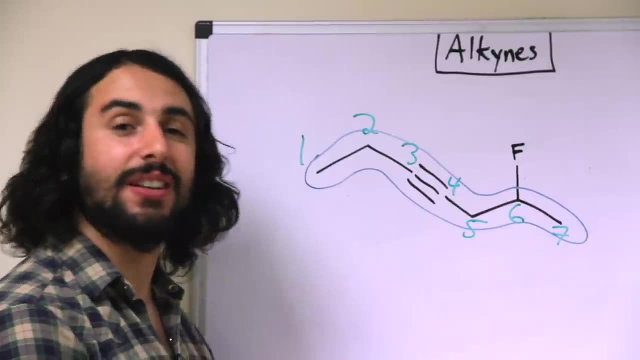 that will give the triple bond occurring soonest. So we do have a 7-carbon alkyne once again, bearing in mind that these are carbon atoms right there and this is the appropriate way to draw an alkyne- a very common error. 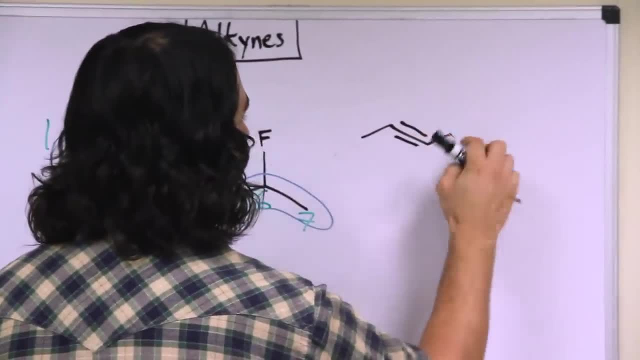 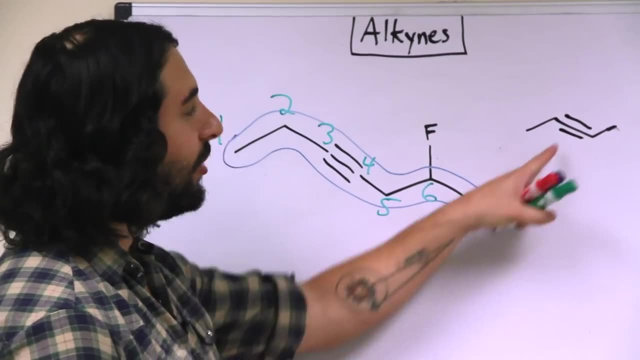 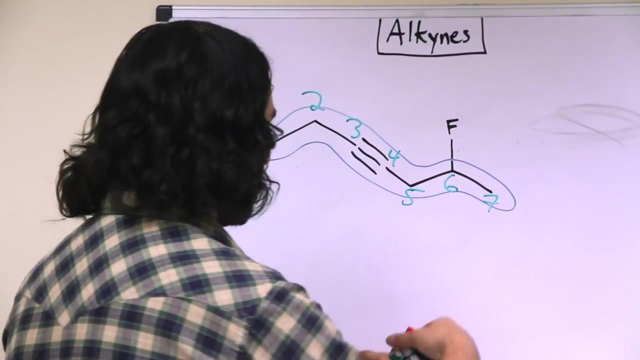 I'll see, is alkynes drawn like that? While you may still be able to provide or interpret the correct IUPAC name for the molecule, this is geometrically incorrect, so we prefer not to draw it that way. So now we just have to identify the substituent. We have a fluoro group. 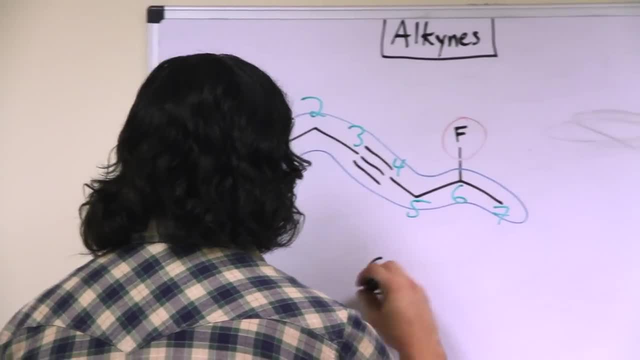 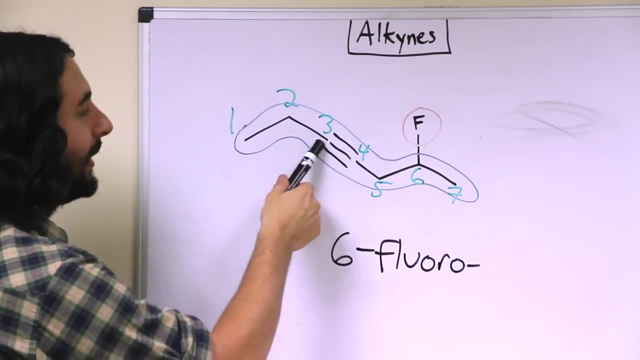 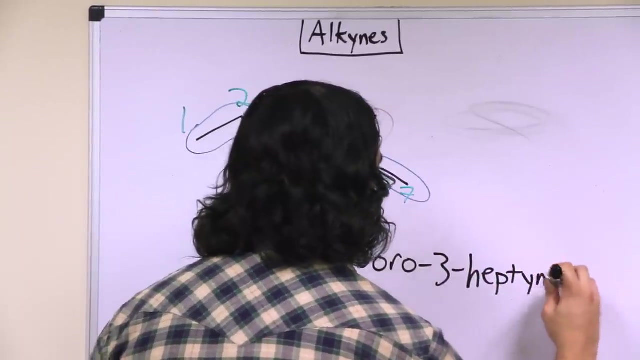 on carbon 2, or, sorry, carbon 6.. So 6, fluoro. and then we must state the location of the triple bond. It begins on carbon 3.. So we have a 3 heptine. So up until this point we've been looking at some pretty simple examples. 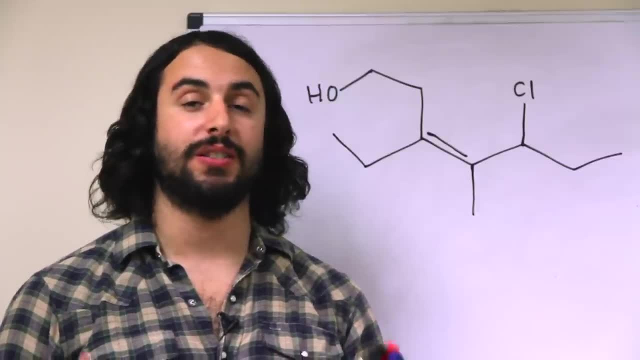 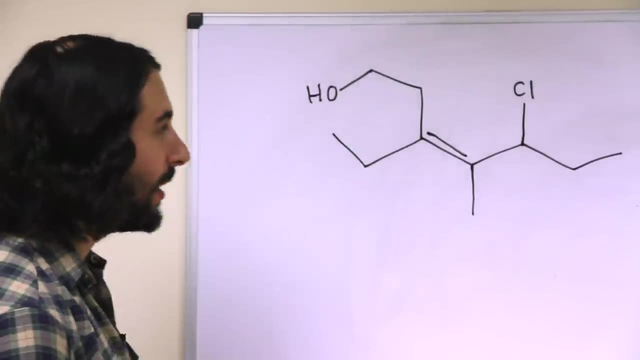 but in reality a lot of organic molecules have multiple different kinds of substituents and different functional groups on the molecule. So let's look at a slightly trickier example and see what happens when we have multiple different kinds of substituents on the molecule. So the first: 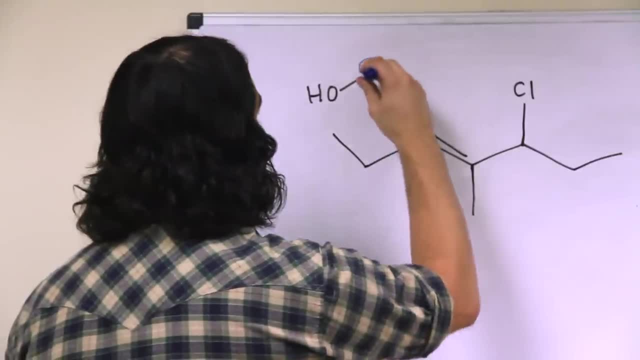 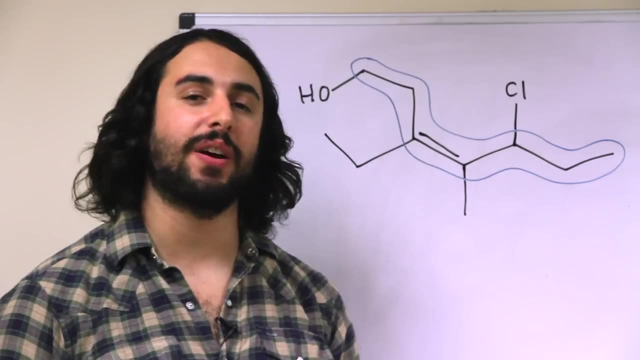 thing we have to do, as always, is identify the longest carbon chain. Now, what we have to keep in mind is that there is an order of prioritization of these functional groups that we need to consult, So of the groups that we've learned, so 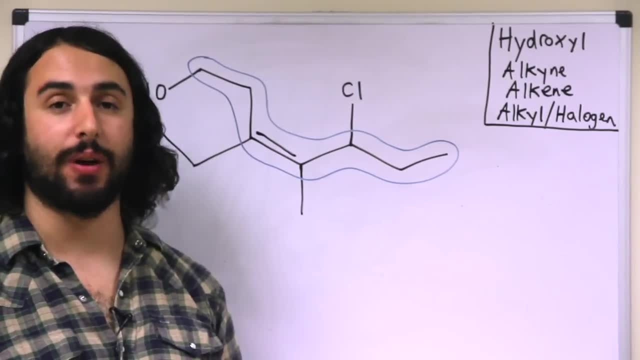 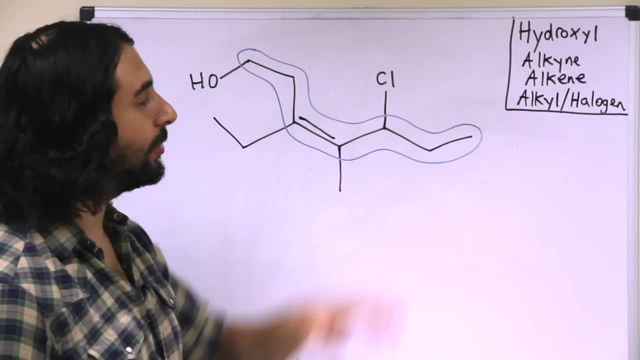 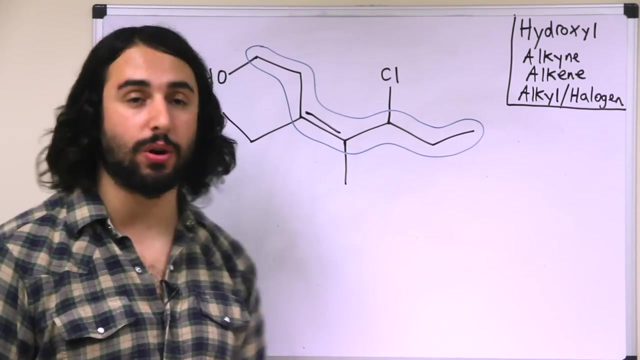 far, this is the priority. The hydroxyl takes top priority. after that would be an alkyne, so a triple bond, then alkene or any double bond, and then alkyl groups and halogen substituents have the same priority. So in this case, because hydroxyl takes the highest priority, it is the 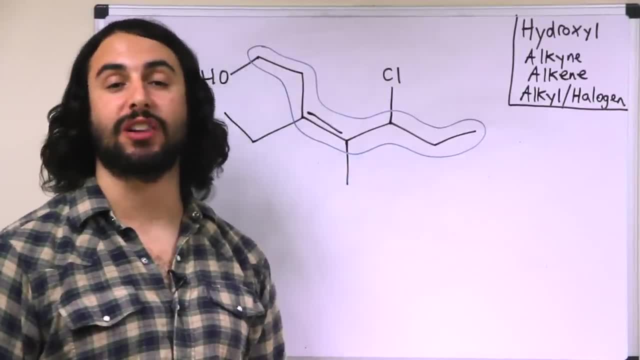 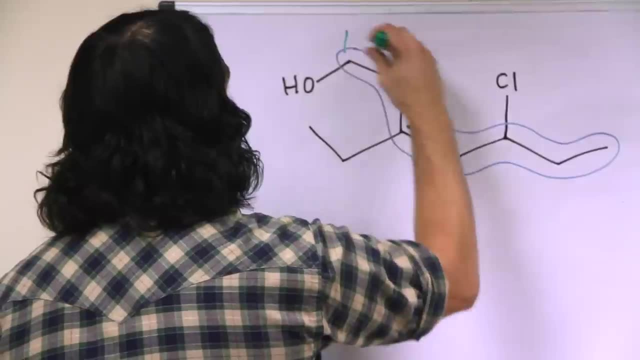 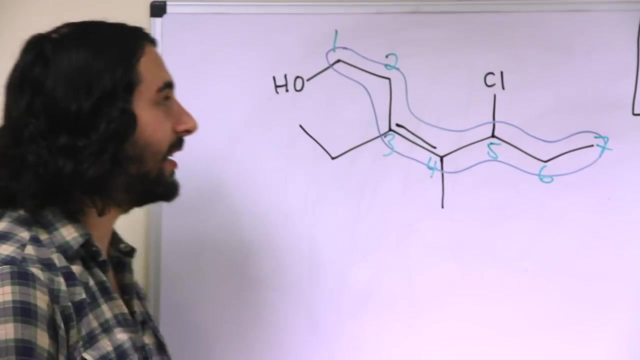 location of the hydroxyl group. that is going to determine the direction that we number this parent chain in. So because the hydroxyl is over here, we must number this left to right. So we have a 7 carbon chain with the hydroxyl on carbon 1.. Now here's another tricky thing. We 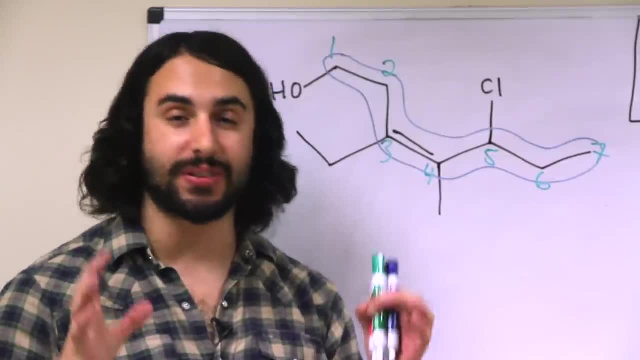 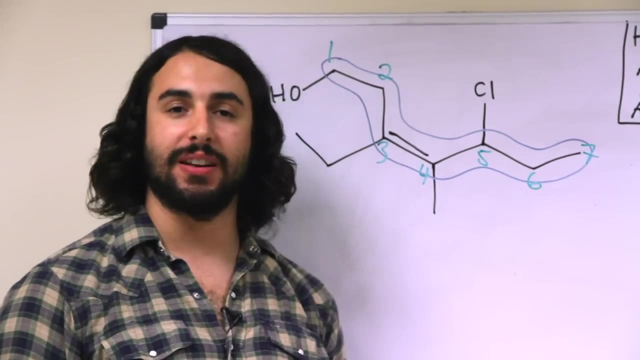 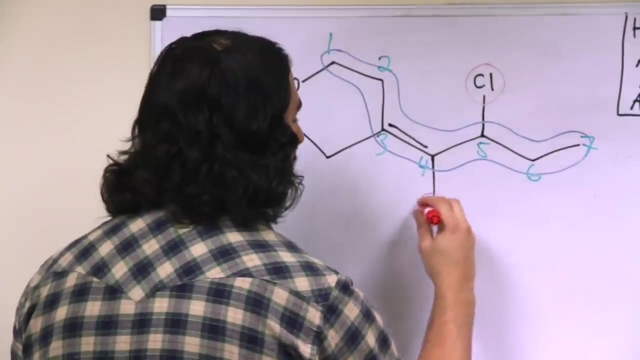 we have two substituents that are both attempting to modify the suffix of the molecule, because this is an alcohol, but it is also an alkene. So that's going to make things a little bit tricky to name, but we do have a way to do it. So let's see what we have. We have got a chloro group, we have got a. 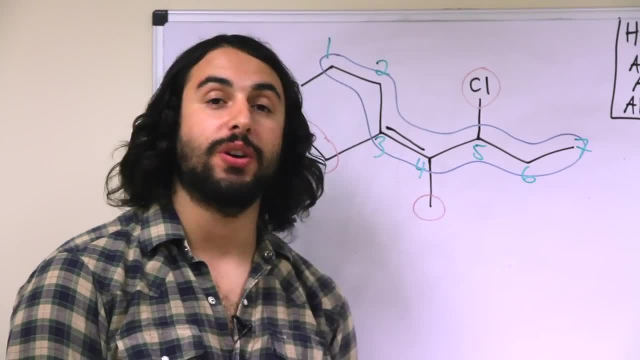 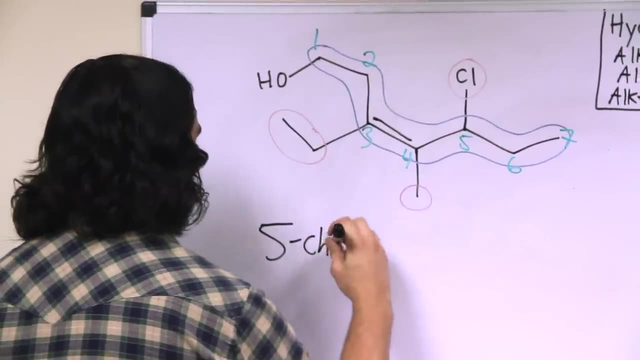 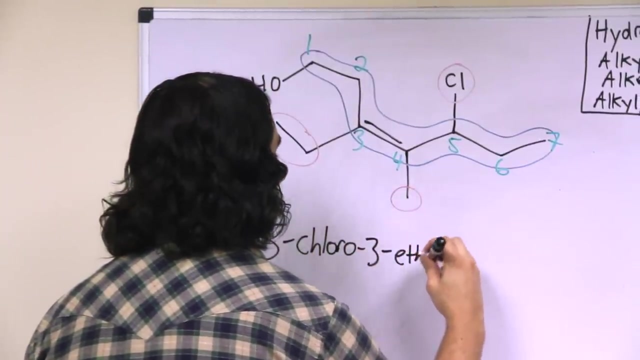 methyl group and we've got an ethyl group. So we're going to list the chloro group first, because C for chloro. So that is five chloro groups, And then we have three ethyl And then we have four methyl. 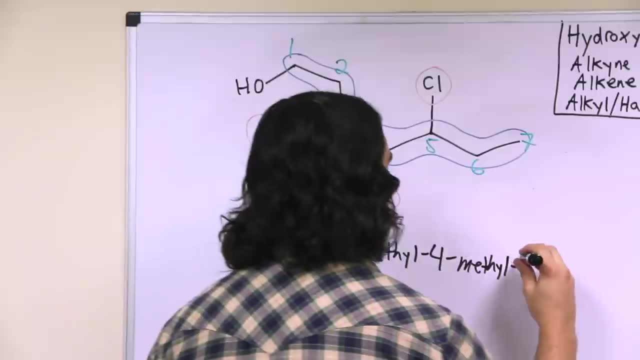 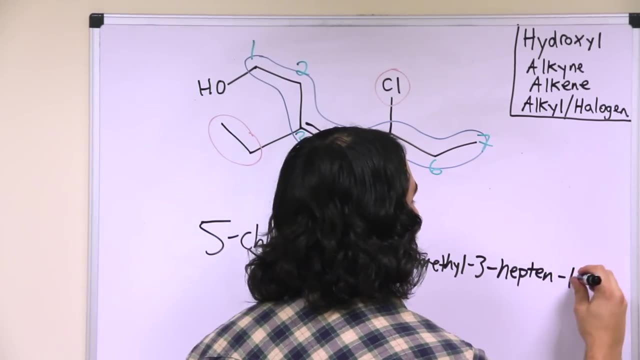 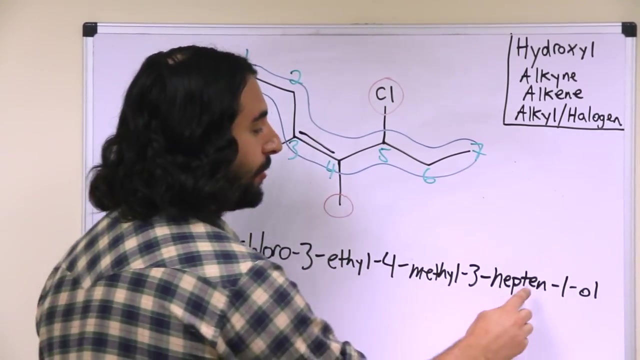 And then here's the kicker: We're going to go three, hepten one all. So this seems a little bit strange, but it has to be done this way, because both the this E is very important because it is indicative of a double bond, and the OL is. 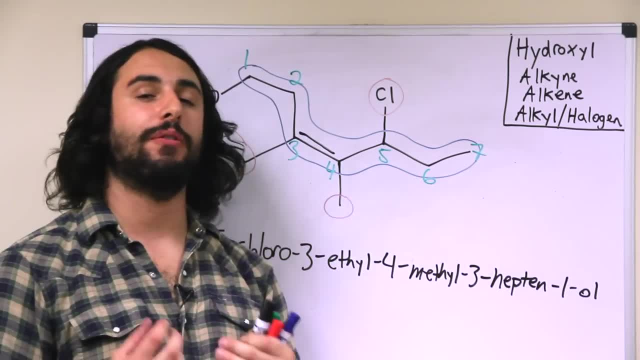 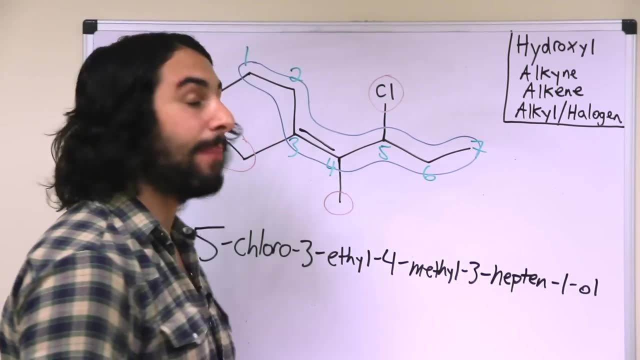 important because it is indicative of the hydroxyl group. But both of those are suffixes at the end of the molecule, so they both have to be there. The convention is to drop the E in heptene to indicate that there is more of the molecule to list and then after that list the presence of 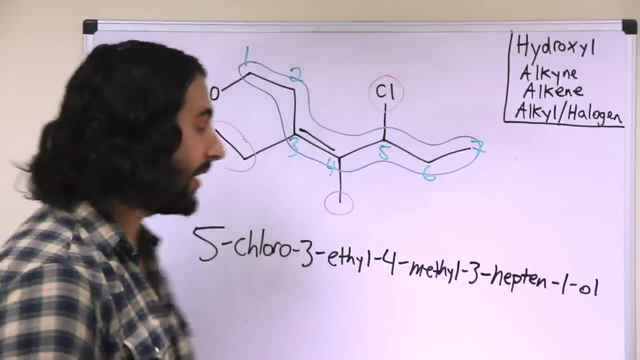 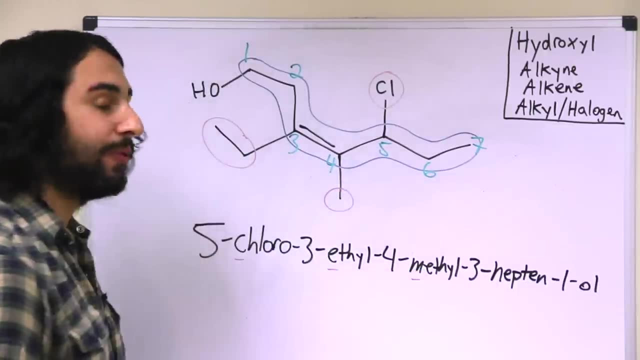 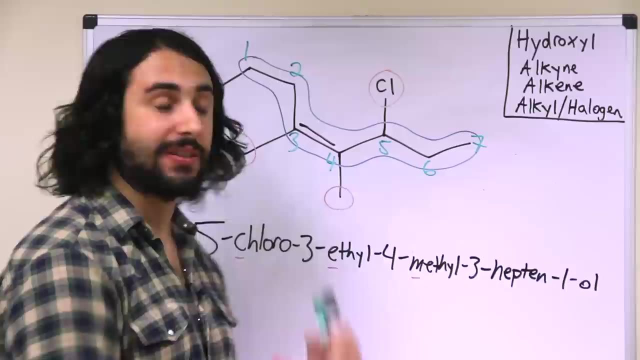 the hydroxyl group last, because that does take the top priority. So once again, the the simpler substituents, your halogens and your alkyls go first, in alphabetical order, and then always last is or are the functional groups that are modifying the suffix of the molecule In this. 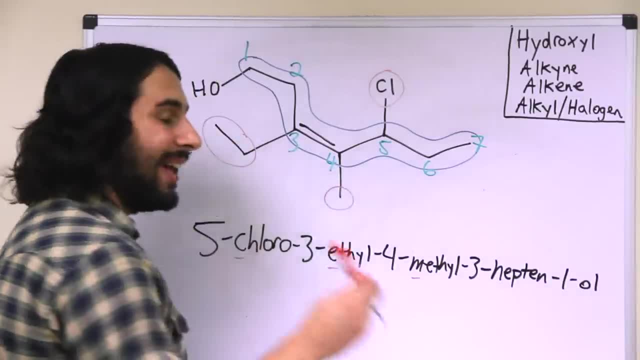 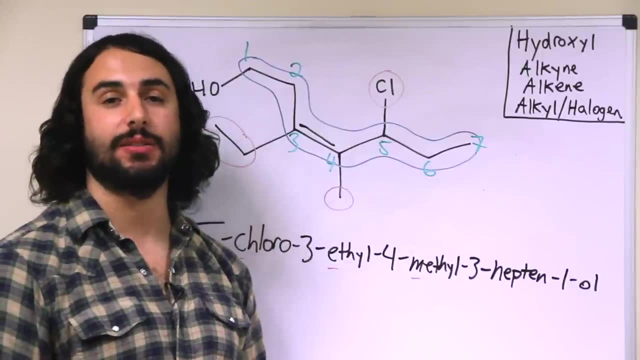 case the presence of the double bond and the hydroxyl, and we do have to list numbers indicating where they occur. otherwise it would be ambiguous as to their location on the molecule. Thanks for watching, guys. Subscribe to my channel for more tutorials and, as always, 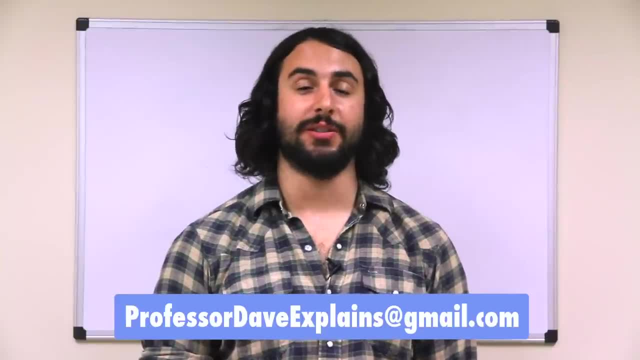 feel free to email me if you have questions, ProfessorDaveExplains at gmailcom.